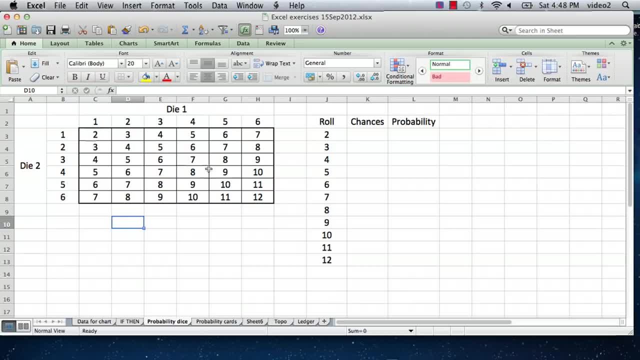 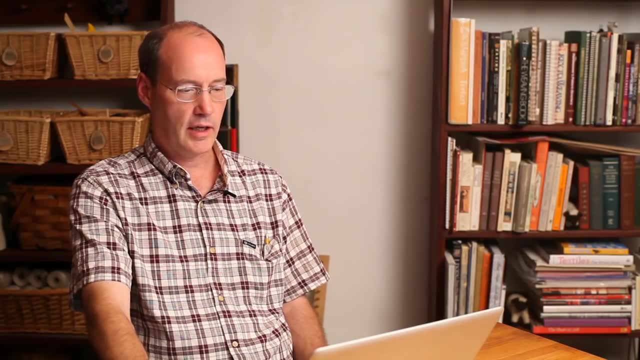 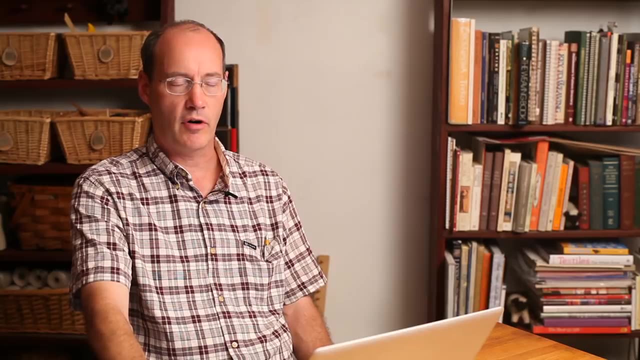 number in column B And I'm going to use those numbers, I'm going to use this little table to calculate the probabilities over here. So any probability is just the number of chances, the number of ways that something can happen, divided by the number of all the different. 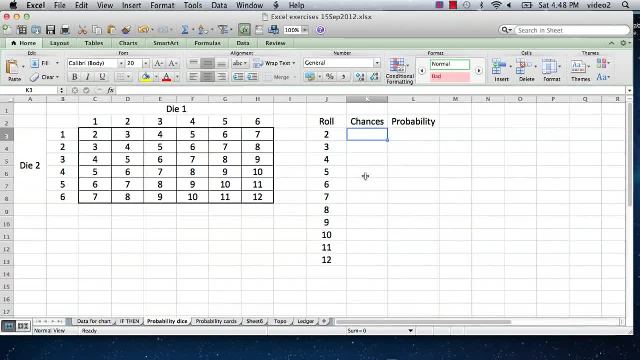 things that can happen, So the number of chances, and that means the number of ways that you can roll the number 2.. We're going to put a formula in here and it's going to be a formula called COUNTIF. So we're going to say equals COUNTIF, and then we're going 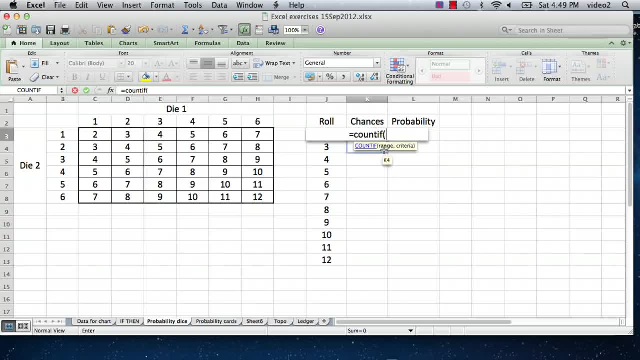 to have in parentheses. it's some of the newer versions of Excel. It's really nice because when you start typing in a formula, it tells you what you want to enter in. So the first thing we want to enter in is the range. That's all the things we want to count. So I'm going. 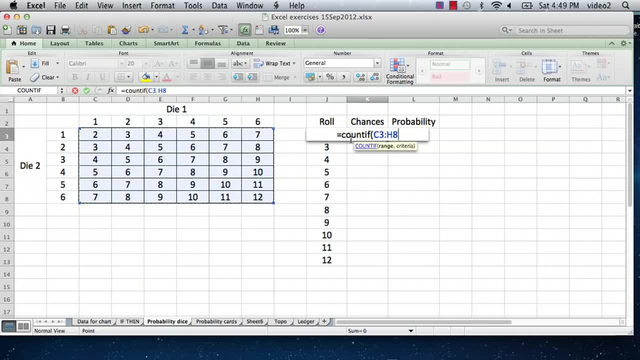 to just draw a box around those 36 numbers in my table. And the other thing I'm going to do- if you've used Excel a little bit, you'll know this is very important- is I'm going to put dollar signs before all the letters and numbers specifying the range, and that. 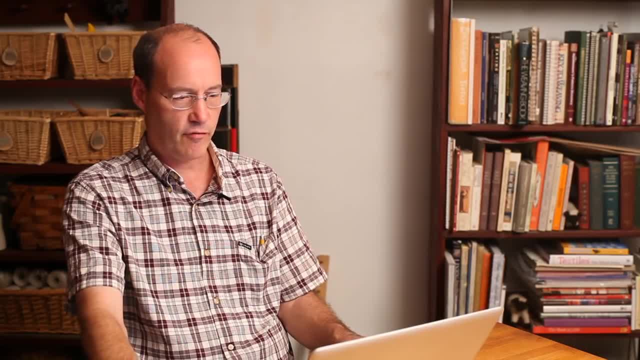 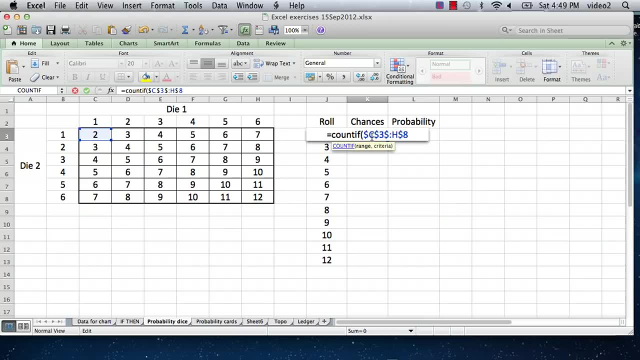 will tell me, tell Excel, that when I copy that formula, those numbers, those references, are not to be changed, because we always want to count with that same box of 6x6.. Oops, and I forgot to type the rest of the formula. 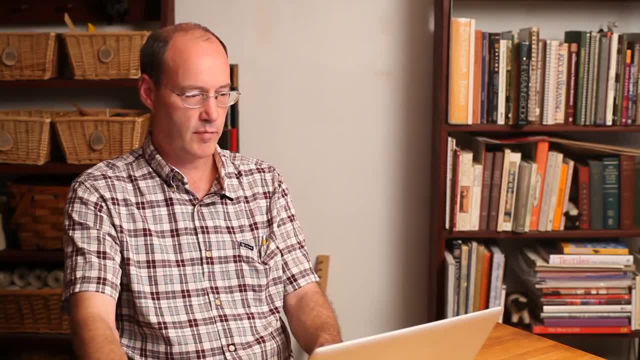 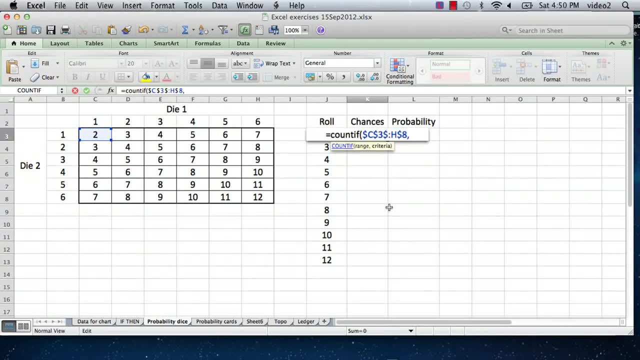 So the next thing that it's looking for it's going to be the number of chances, and that's what we're looking for is the criteria, And that just means what it is we want, And we want to count the numbers if it equals the contents of J3, which is where our number 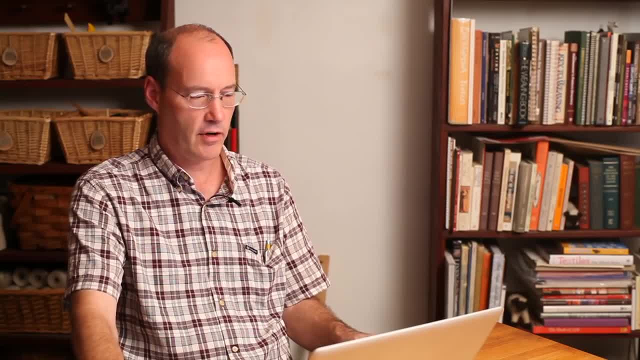 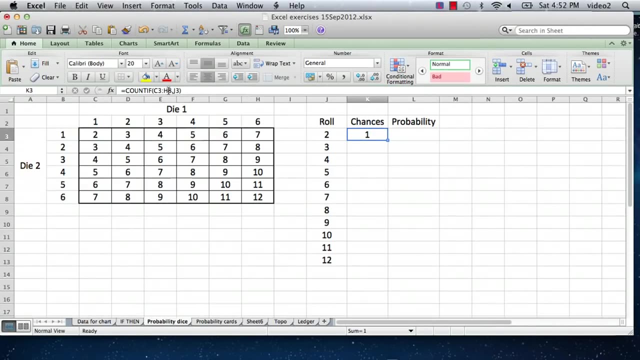 2 is. So what this is saying is we're going to count all of the number of cells in the range C3 to C8 where the value equals 2.. So we want basically all the ways in which that we can roll 2 with the dice. Now, one thing we want to do before we copy this formula: 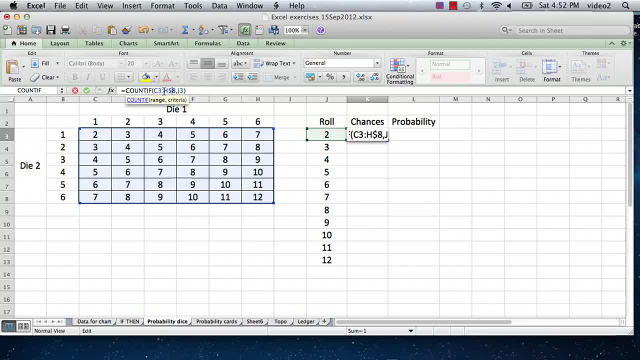 is go up into the formula and put dollar signs before all the letters and numbers in the range, because we don't want it to change when we copy the cell, when we copy the formula. So there we go. Now we're just going to go to the bottom right of this cell and drag. 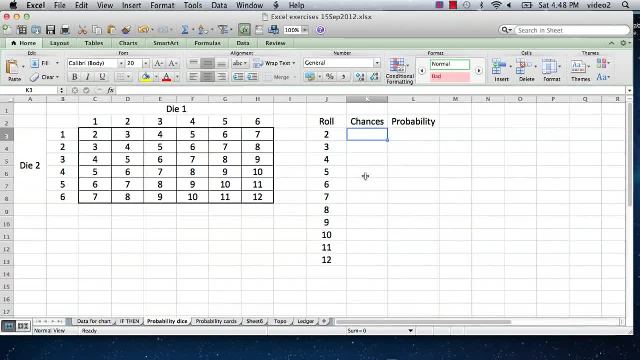 things that can happen, So the number of chances, and that means the number of ways that you can roll the number 2.. We're going to put a formula in here and it's going to be a formula called COUNTIF. So we're going to say equals COUNTIF, and then we're going 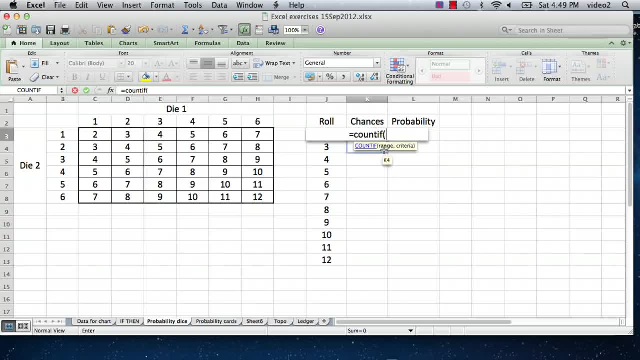 to have in parentheses. it's some of the newer versions of Excel. It's really nice because when you start typing in a formula, it tells you what you want to enter in. So the first thing we want to enter in is the range. That's all the things we want to count. So I'm going. 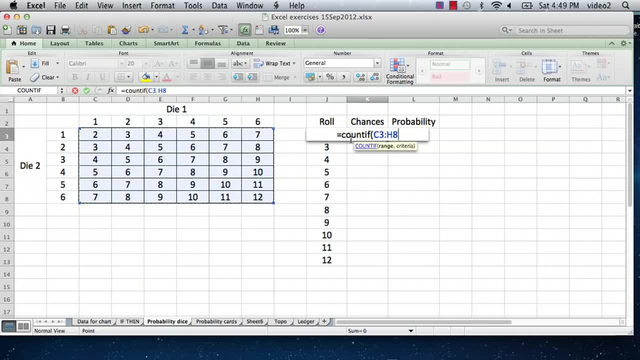 to just draw a box around those 36 numbers in my table. And the other thing I'm going to do- if you've used Excel a little bit, you'll know this is very important- is I'm going to put dollar signs before all the letters and numbers specifying the range, and that. 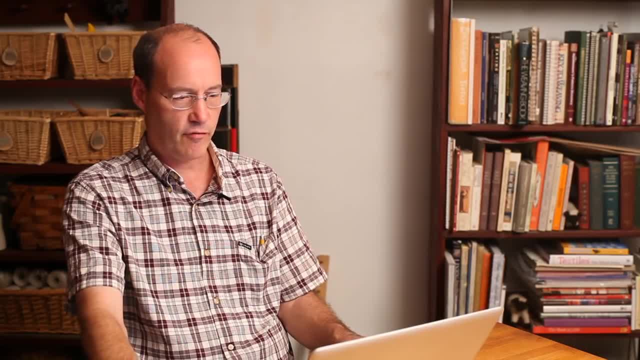 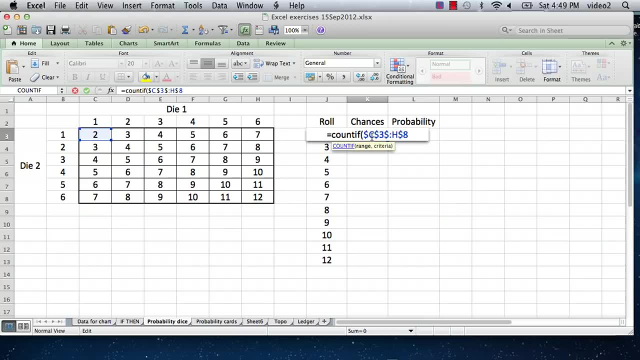 will tell me, tell Excel, that when I copy that formula, those numbers, those references, are not to be changed, because we always want to count with that same box of 6x6.. Oops, and I forgot to type the rest of the formula. 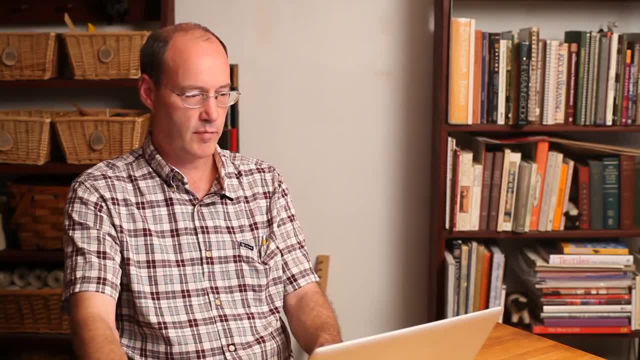 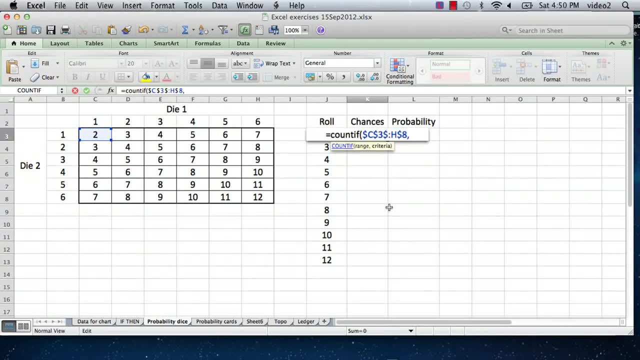 So the next thing that it's looking for it's going to be the number of chances, and that's what we're looking for is the criteria, And that just means what it is we want, And we want to count the numbers if it equals the contents of J3, which is where our number 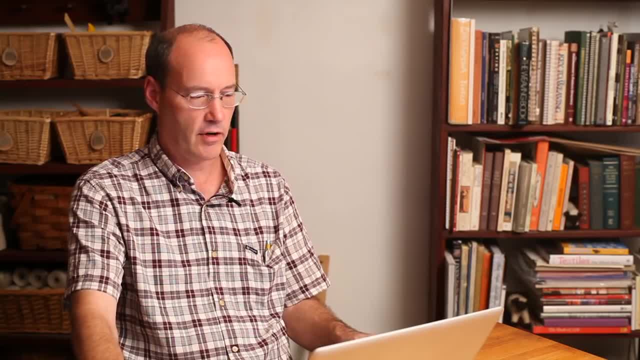 2 is. So what this is saying is: we're going to count all of the number of cells in the range C3 to C8 where the value equals 2.. So we want basically all the ways that we're going to count the number of cells in the range C3 to C8 where the value equals 2.. Now 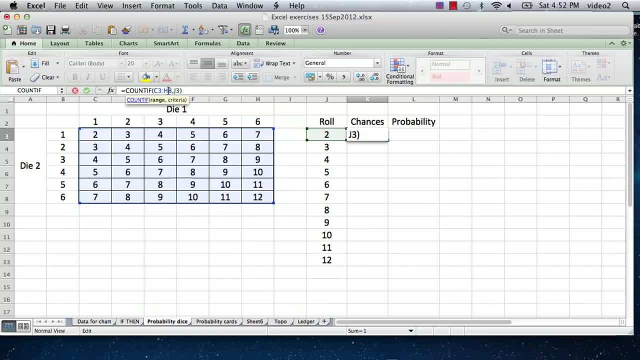 one thing we want to do before we copy this formula is go up into the formula and put dollar signs before all the letters and numbers in the range, because we don't want it to change when we copy the cell, when we copy the formula. 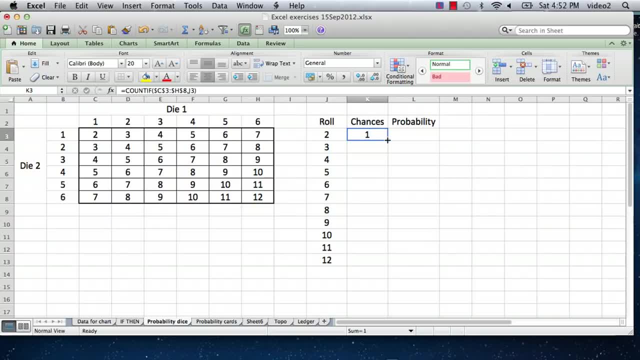 So there we go. Now we're just going to go to the bottom right of this cell and drag it down, and that just copies the formula to all the other lines with the corresponding where it counts, the number: 1,, 2,, 3,, 4,, 5,, 6,, 7,, 8,, 9,, 10,, 11,, 12,, 12,, 13,, 14,, 15,, 16,, 17,, 18,. 19,, 20,, 21,, 21,, 22,, 23,, 24,, 25,, 26,, 27,, 28,, 29,, 30,, 31,, 32,, 34,, 35,, 35,, 36,, 37,, 38,, 40,. 42,, 47,, 42,, 48,, 42,, 45,, 40,, 42,, 45,, 46,, 47,, 48,, 42,, 45,, 46,, 47,, 49,, 49,, 50,, 94,, 51,, 52,.